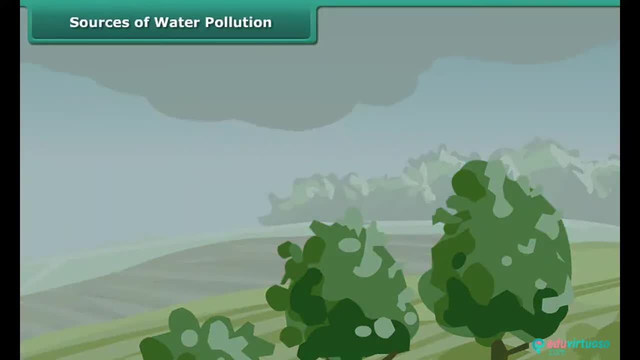 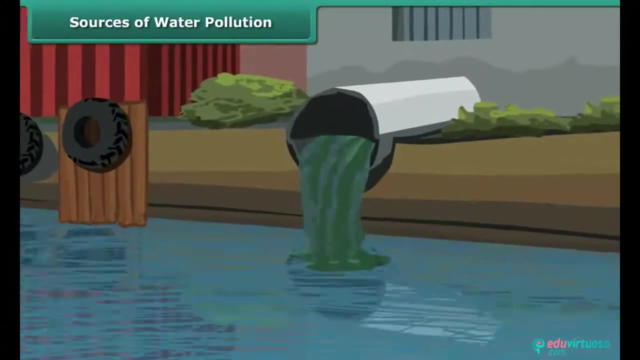 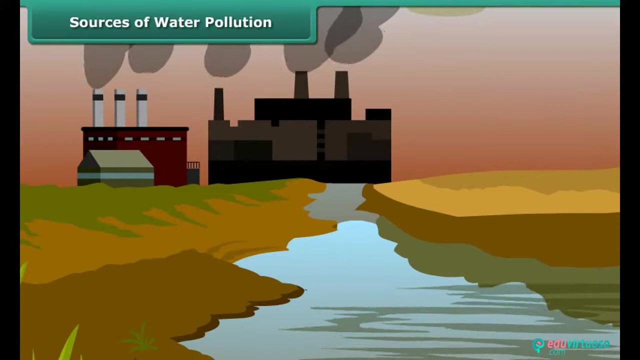 eroded soil runoff containing fertilizers and pesticides as chemicals released from industries and other waste from cities and towns. The chemicals released from industries, like arsenic lead and fluorides, lead to toxicity in plants and animals. Often, the factories and power plants use normal. 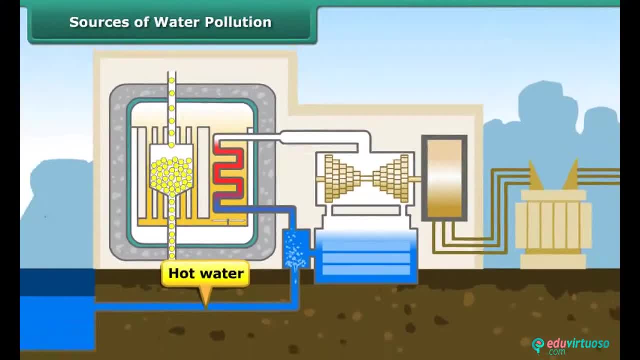 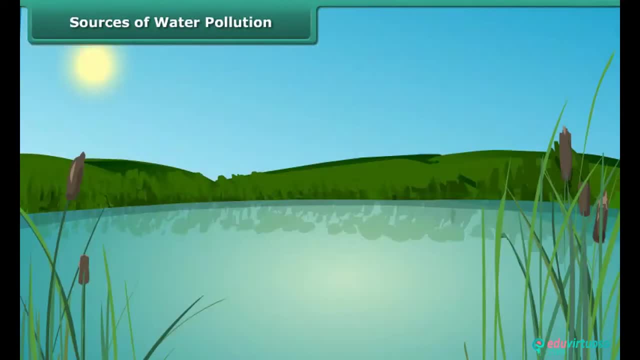 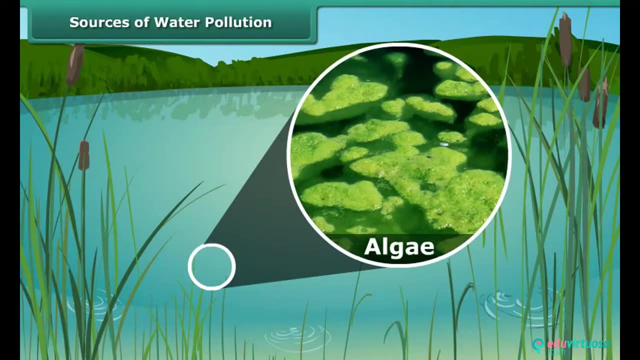 water to cool their machinery and then release hot water. It heats up the water body and aquatic animals die in it. Have you seen ponds which look green from a distance? This is due to algae grown in it. Do you know how these algae grow in the pond? 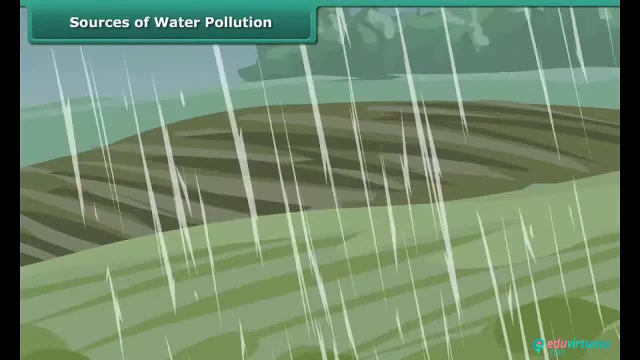 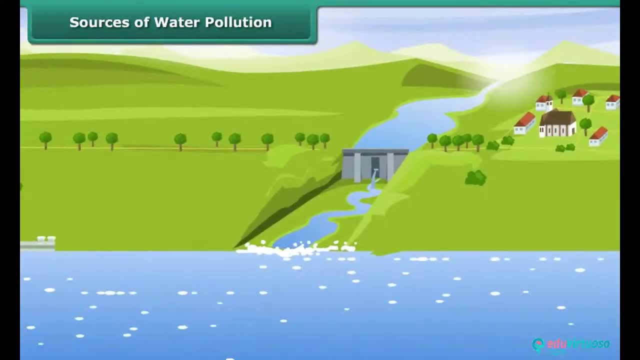 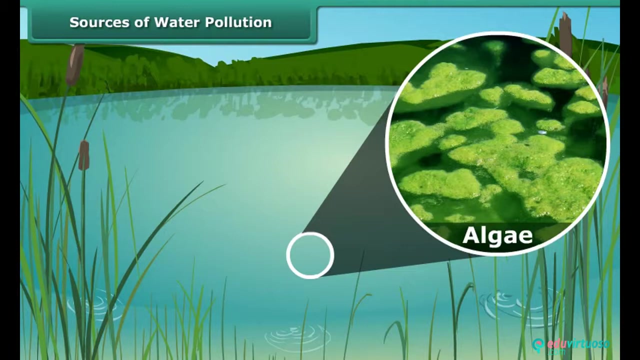 During rainfall, large amounts of fertilizers get washed from the fields and fall on the ponds and rivers. These washed off fertilizers act as nutrients for algae to flourish. When these algae die, they serve as food for the decomposers, like bacteria. 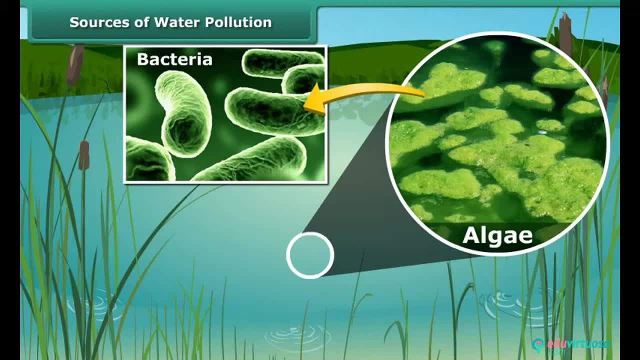 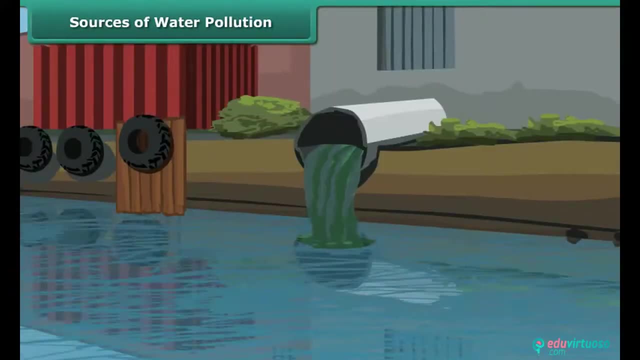 Bacteria use up most of the oxygen in the water and, as a result, the fish and other aquatic animals die due to lack of oxygen. Also, people bathe, wash clothes and defecate in the rivers and ponds. They also throw. 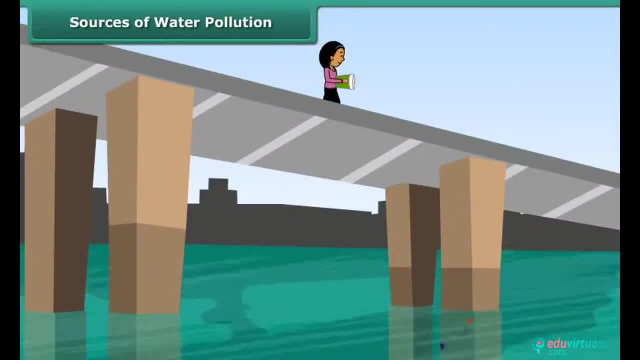 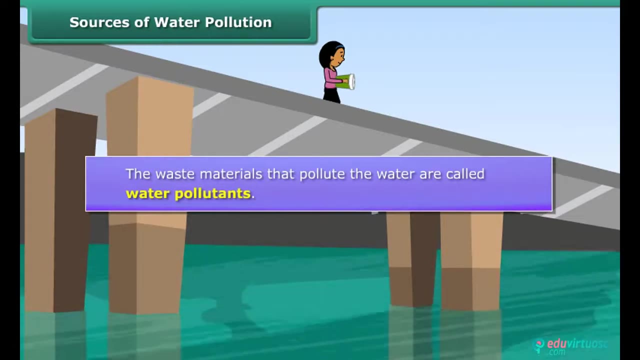 garbage flowers and non-biodegradable polythene bags into the river. Many rivers have become dead due to a high level of pollution, and aquatic life cannot survive in them. The waste materials that pollute the water are called water pollutants. Let us check. 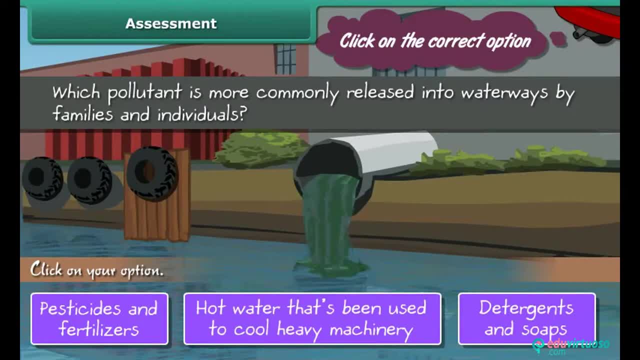 your understanding on the topic covered. How much water does water produce? The water that is used in the water is about 1.5 tons per liter. The amount of water is about 50 tons per liter. The amount of water is about 2 tons per liter. 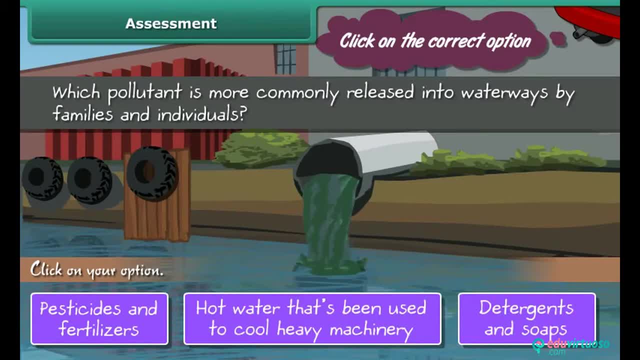 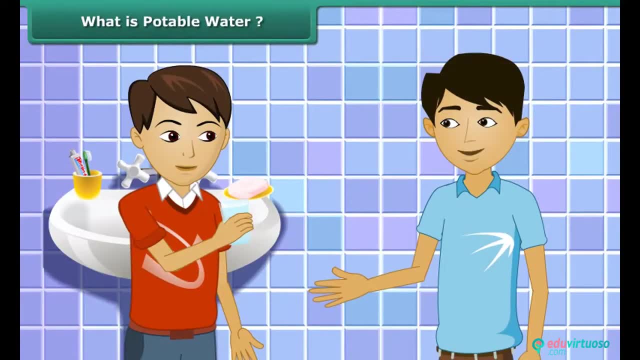 The amount of water is about 3 tons per liter. In other words, the amount of water is about 6 tons per liter. What are you doing? why it is clean water? water that looks clean may still have disease, carrying microorganisms and dissolved impurities, which can cause illness. really, yes, you.